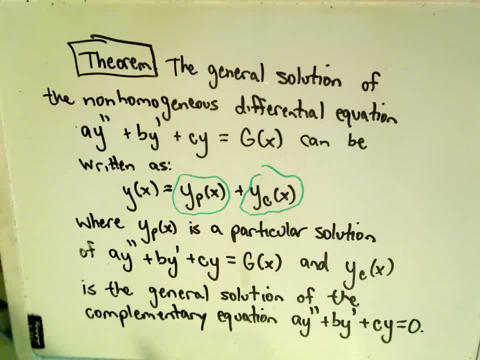 And y of c is going to be a solution to the complementary equation that we're trying to solve. Okay, so let's try to make some sense out of all this. Solving this last part isn't too bad. I mean, you just have to remember some of the other formulas for. 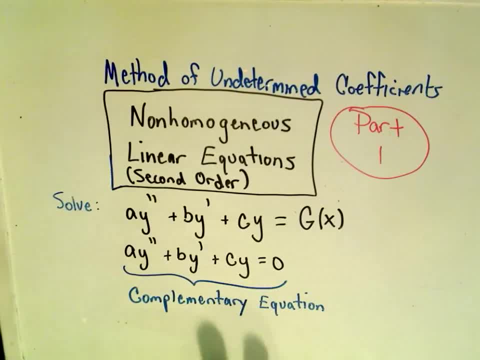 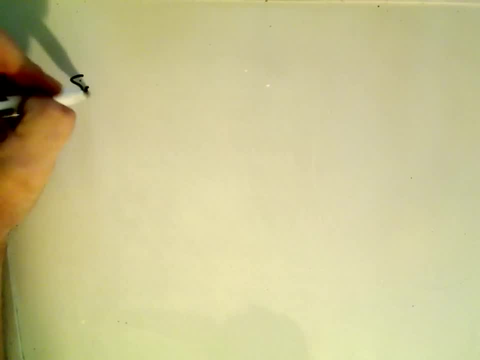 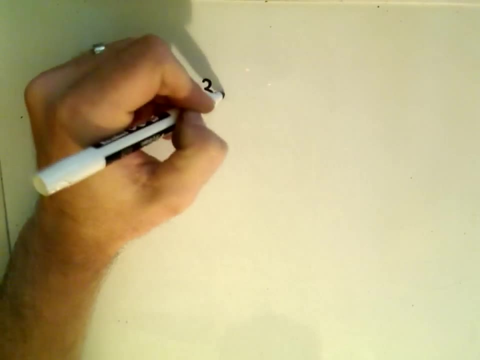 Okay, Differential equations, but hopefully not too bad to start off with. Okay, so let's solve this corresponding. let's try to solve this. So we're going to have y double prime plus 3y, prime plus 2y equals x squared. 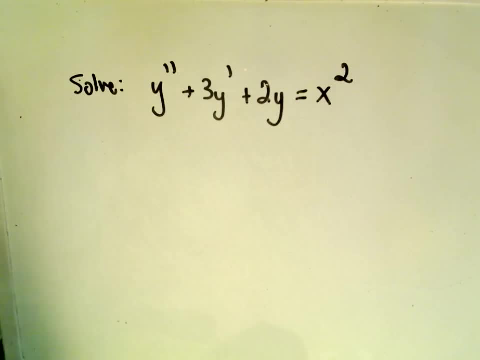 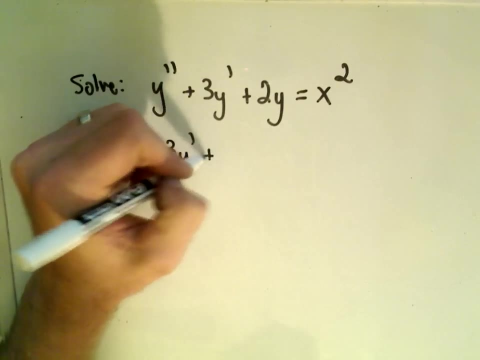 Okay. so the first thing, what we're going to do again, is just turn this into our complementary equation And we're going to solve first off. So we're going to have y double prime plus 3y prime plus 2y equals 0.. 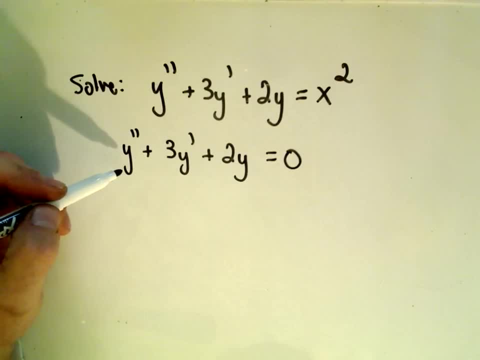 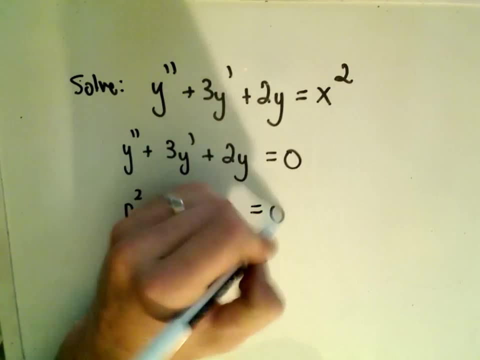 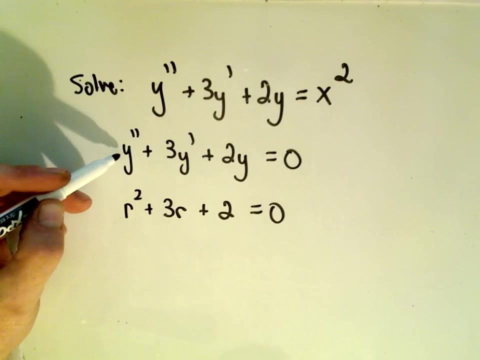 Okay, Now we turn this into what's called the auxiliary equation: r squared plus 3r plus 2 equals 0.. And then, based on the solutions to this auxiliary equation, it's going to tell us solutions to our homogenous second order differential equation that we have here. 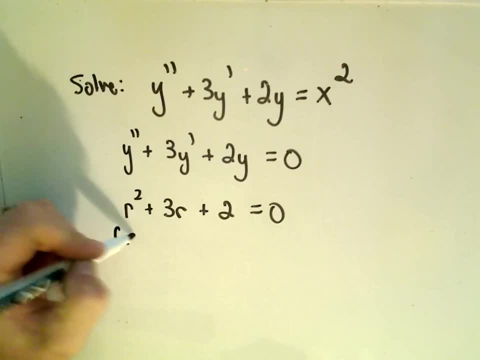 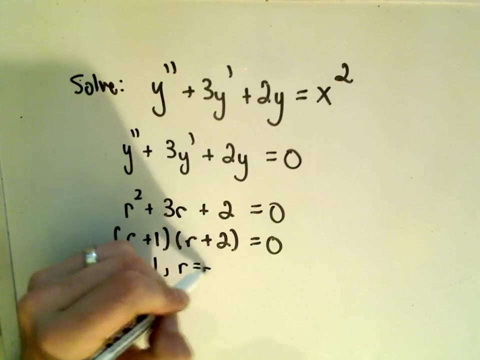 Okay, so I think this is going to factor relatively easily. Looks like we'll just get r plus 1 times r plus 2 equals 0. So that means our solutions are going to be: r equals negative 1 and also r equals negative 2.. 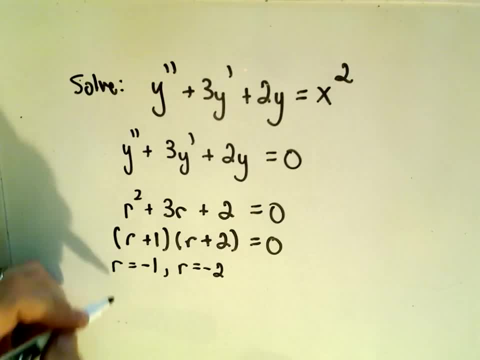 So this is a case where we have two distinct real roots And remember, if you have two distinct real roots, it says, basically, your solution is: It's going to look something like There's going to be some coefficient e to the first root. 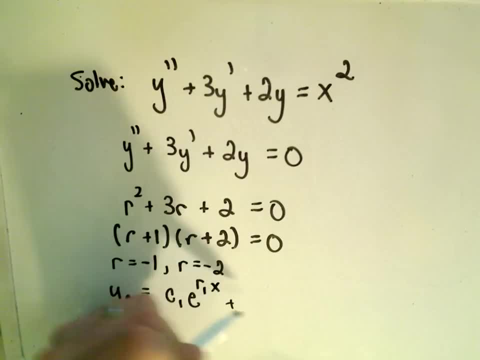 It doesn't matter which one. So one of the roots: times x, plus again this coefficient c2 e to the second root, times x. So okay, well, we know our roots here. All we have to do is plug those in. 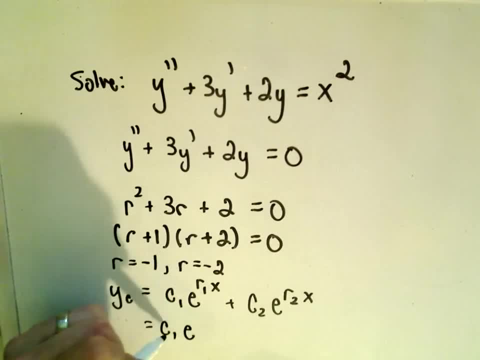 So our general solution is going to be c1 e to the negative x plus c2 e to the negative 2x. Okay, so this is going to incorporate, be incorporated into part of our solution at the end. So, and I think I'm going to stop this part here,